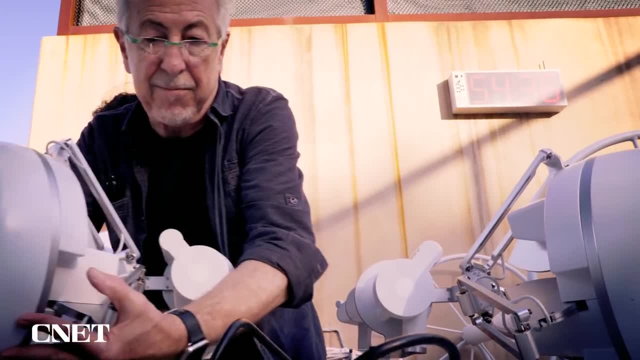 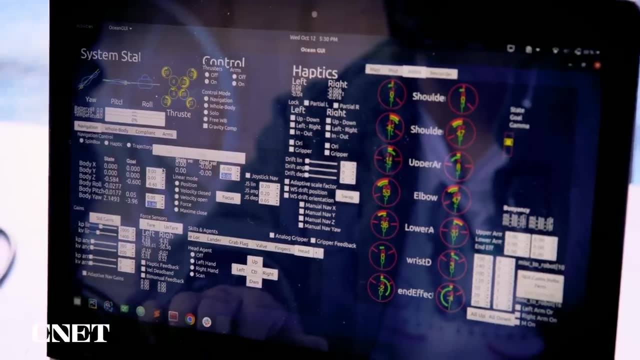 robotics lab. Lab director Usama Khatib wanted to create a robot that could explore the deep ocean using haptics or touch-based controls. The result: A deep-sea robot built tough like a submarine, but with the agility of a human. 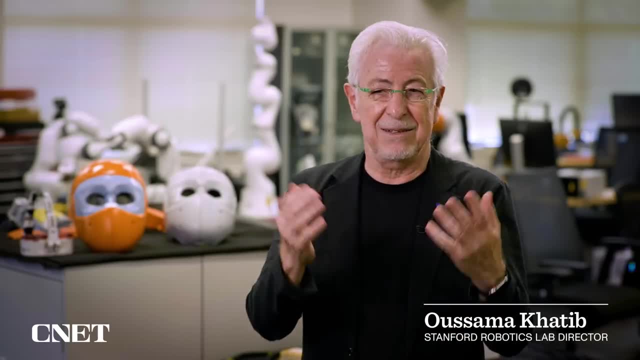 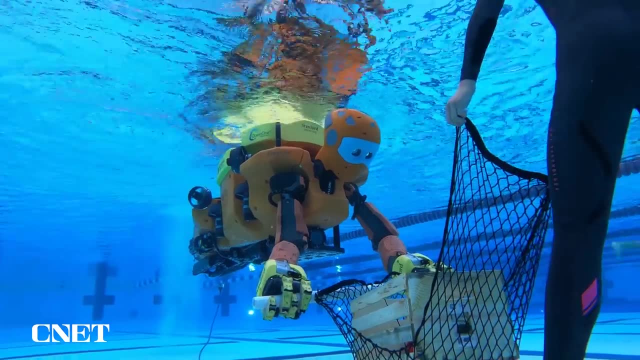 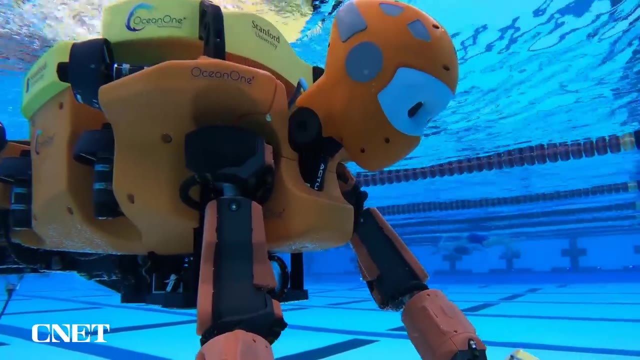 A human cannot dive beyond hundreds of meters. If we need to interact with the environment, with the oceans, we need a machine, And today we have a lot of machines. but these machines can see, but they cannot do, And this is Ocean 1.. Ocean 1, essentially, is your hands, your 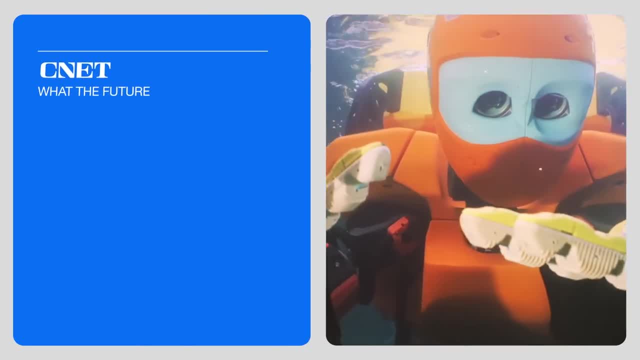 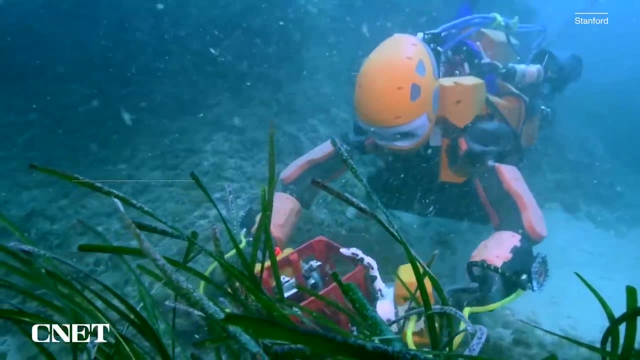 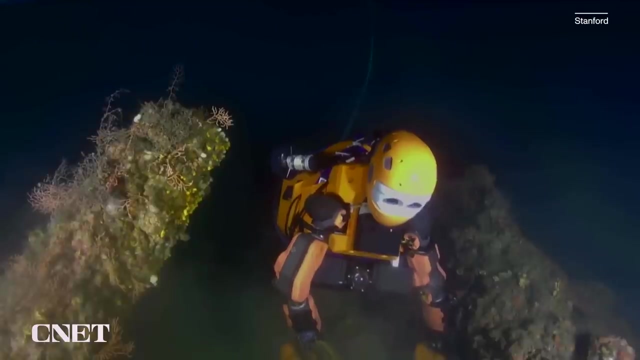 eyes, it's your avatar in the water. The robot started life as a prototype known as the Ocean 1.. Back in 2016,, Stanford took the Ocean 1 down to a 17th century shipwreck off the coast of France. While the design 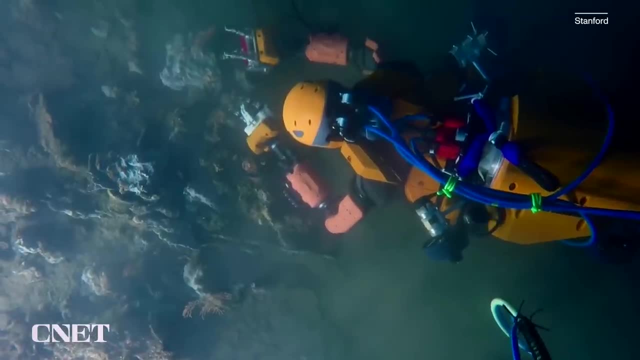 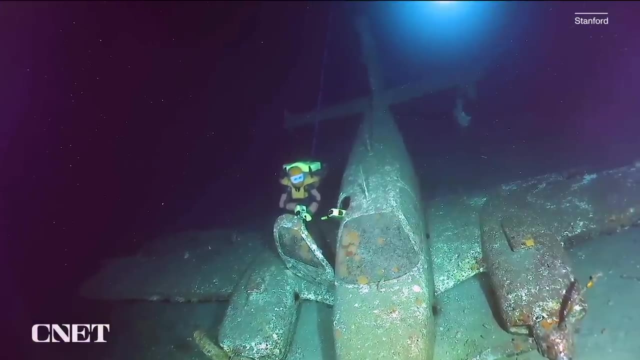 worked, the team realized they needed to be able to go deeper underwater, So Khatib began working on the Ocean 1K, a new, stronger robot that takes its name from the 1000 meters it can go below the surface. 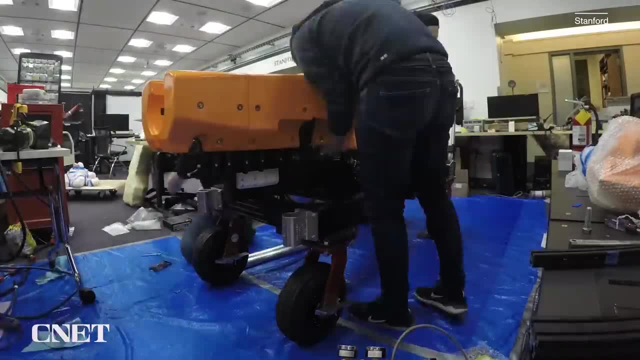 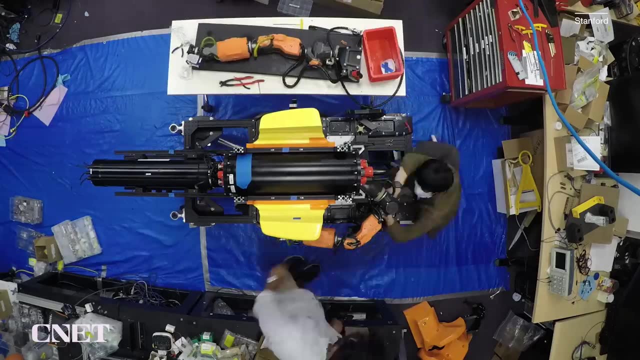 How did it come to be? How did it go? the team had to redesign the robot to survive Going to 1,000 metres. it's almost like 10 times the depth we went to before. This is 100 times the atmospheric pressure. 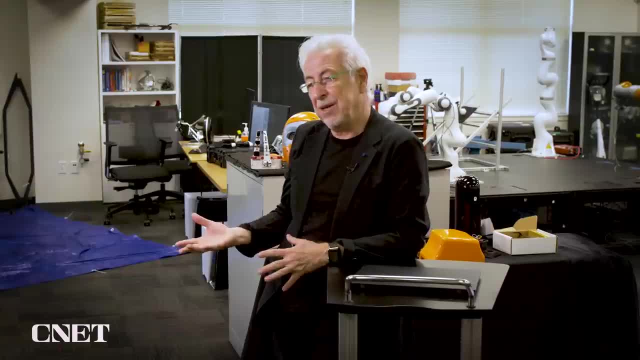 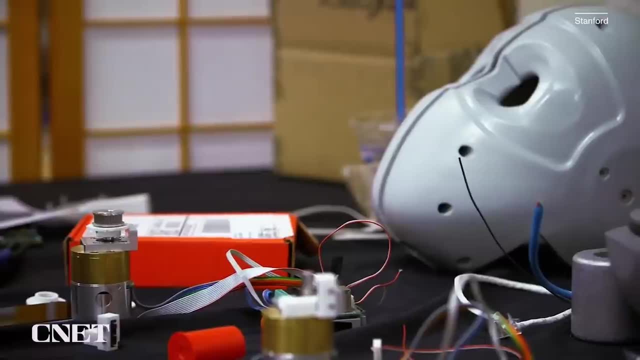 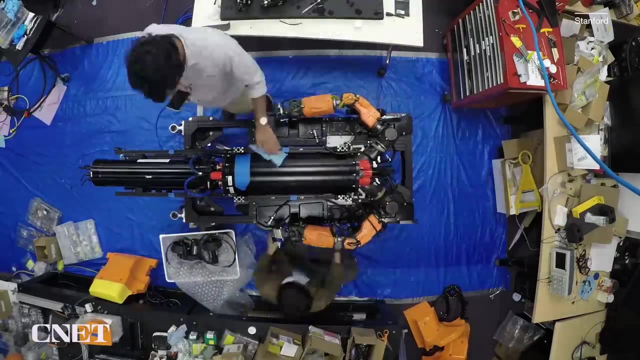 It's a huge pressure And everything we've done before will collapse at that pressure. To help it survive those pressures while still being able to float, Khatib and his team filled the robot's arms with oil. Special spring mechanisms then compressed that oil. 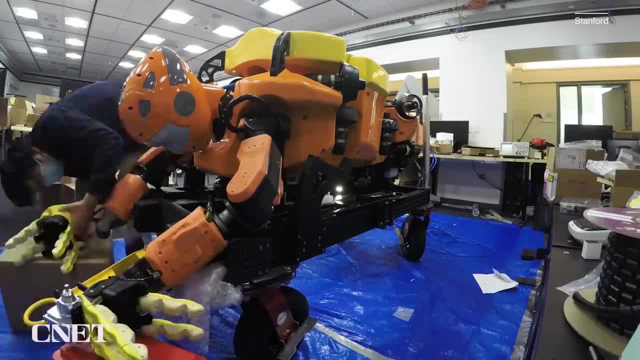 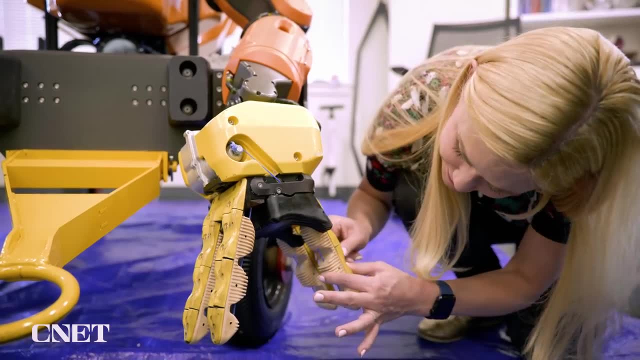 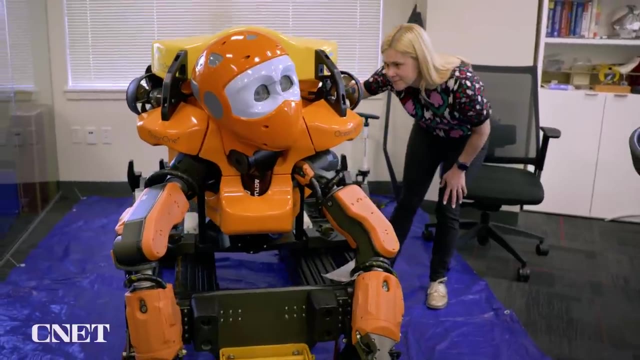 to match the water pressure, stopping the arms from collapsing and protecting the electronics inside. The team also upgraded the robot's hands with more fingers and more grip so it could handle delicate objects underwater. The result is a very human-looking robot, But according to Khatib, 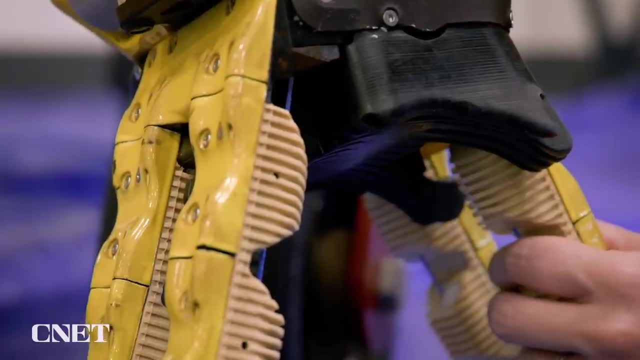 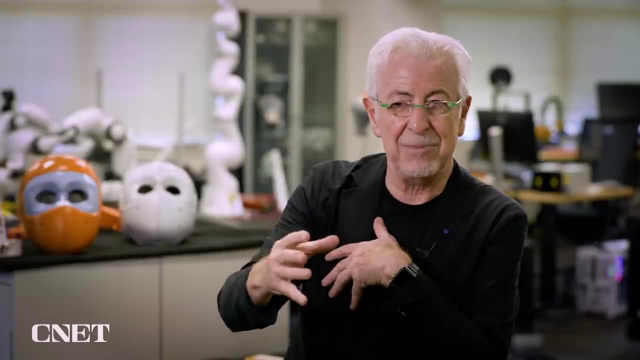 being able to work underwater and pick up things- delicate objects- meant designing a robot with a human shape. In this environment, you cannot work with one arm or one hand. If you put your arm behind your back and think about how you're going to do things, 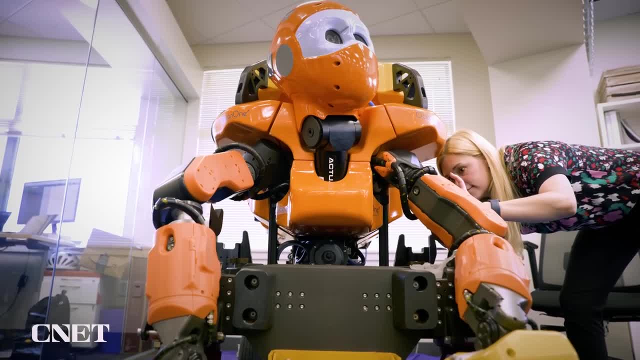 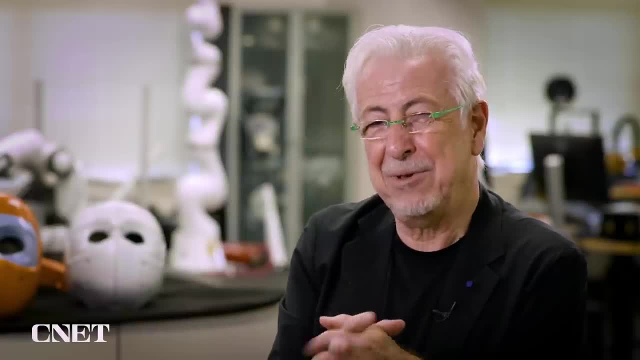 it's very difficult. So you need two arms. Already you get the upper body of a human right. Remember, this is a mermaid, It's not a human-like. We didn't put legs on it. That mermaid is also built with stereoscopic vision. 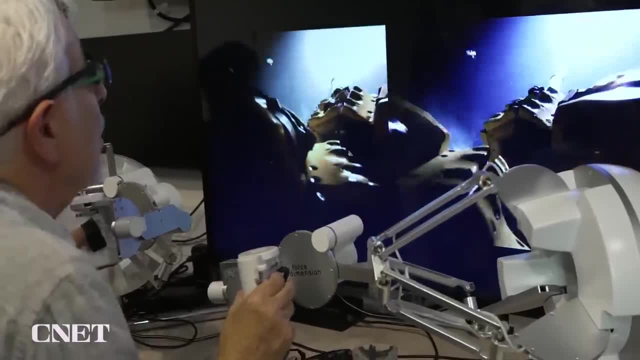 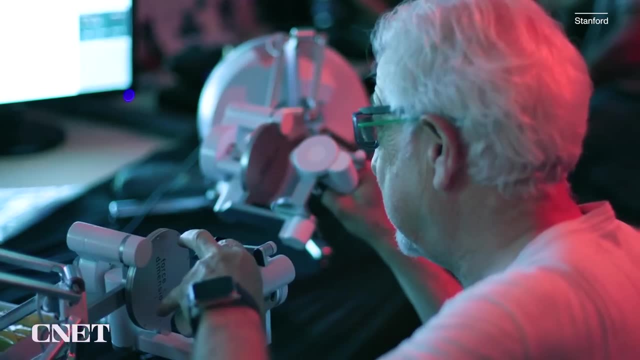 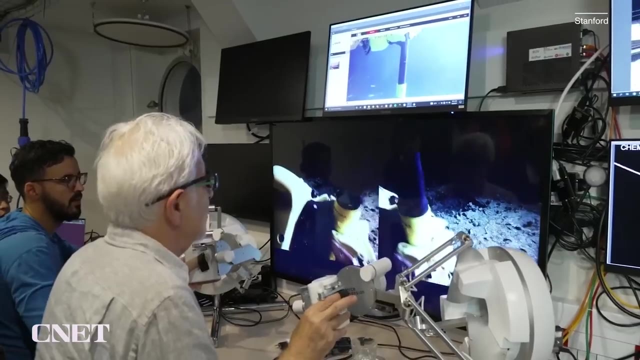 A camera in each eye that creates three-dimensional depth. But the biggest achievement of this robot is the haptics Sensors in the robot's hands that give feedback to the human controller. When the hands hit an obstacle or pick up an object, the human behind the controls can feel it. 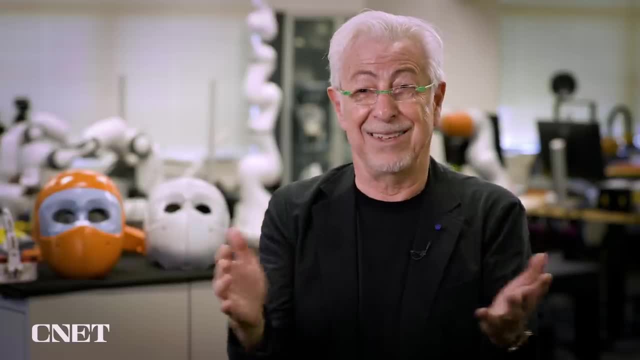 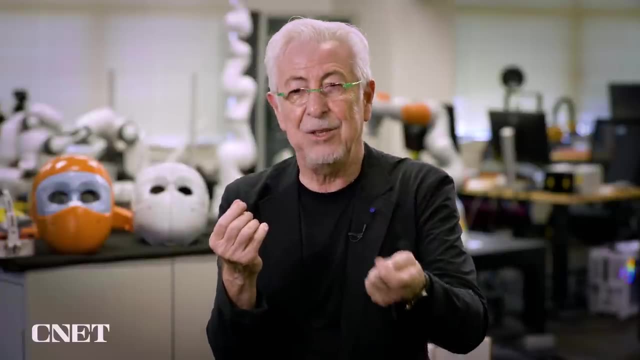 as though they're in the water. Oh my God, this is amazing. I mean, you really feel like you're touching real material. You can feel it. You can feel the friction, the compliance, You can feel everything as if your hand was there. 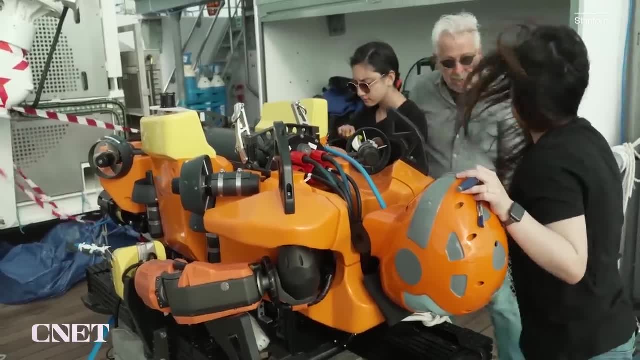 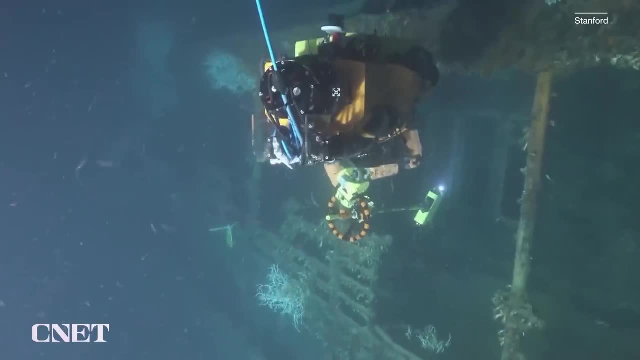 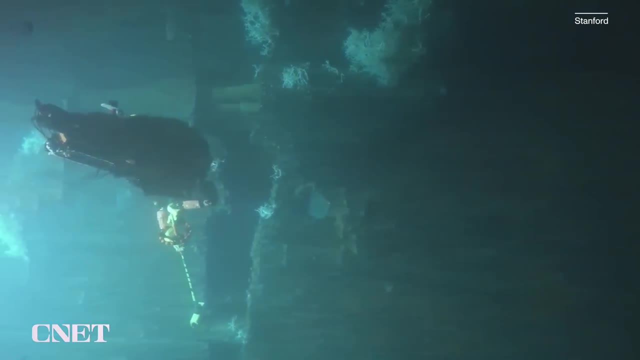 In July 2022, Khatib and his team took the new and improved Ocean 1K to the Mediterranean, testing the robot at different depths. They even used a robot-held camera to get in close to shipwrecks, something that many bulky underwater robots just can't do. 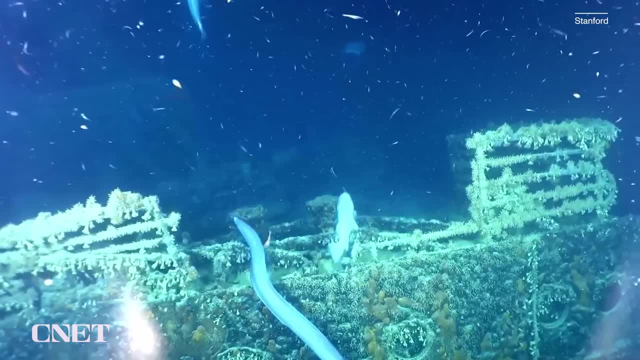 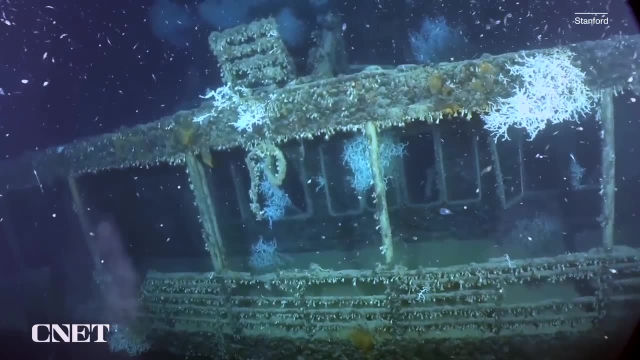 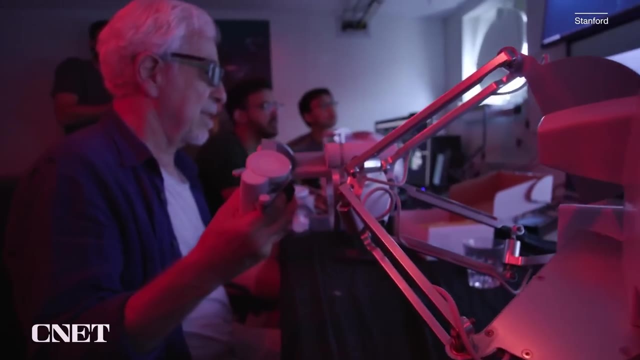 But for Khatib, the highlight was seeing the wreck of an Italian steamship, the Francesco Crispi, 500 metres underwater. Approaching the Crispi was one of the most incredible experiences I've ever had. You are seeing looking through the eyes of the robot. 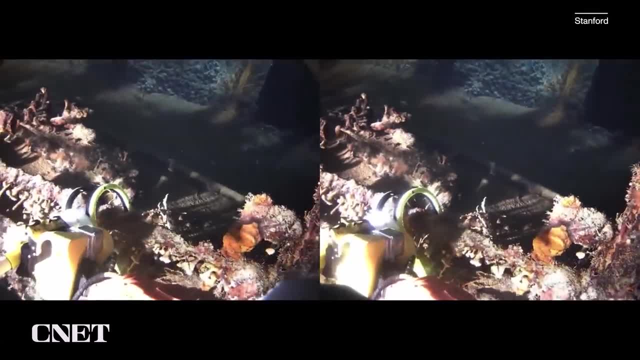 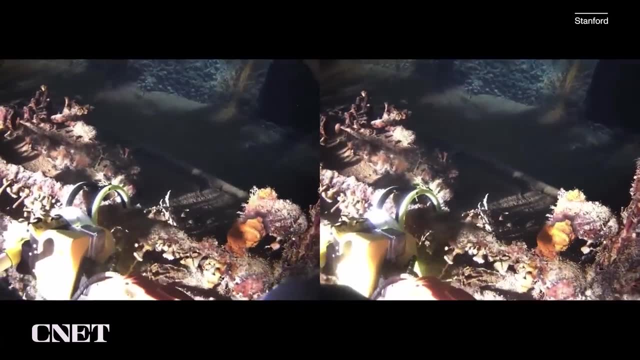 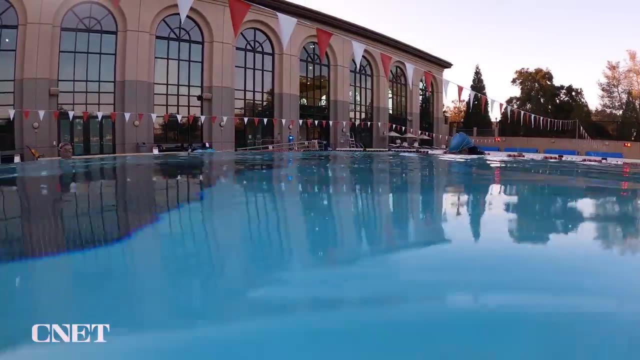 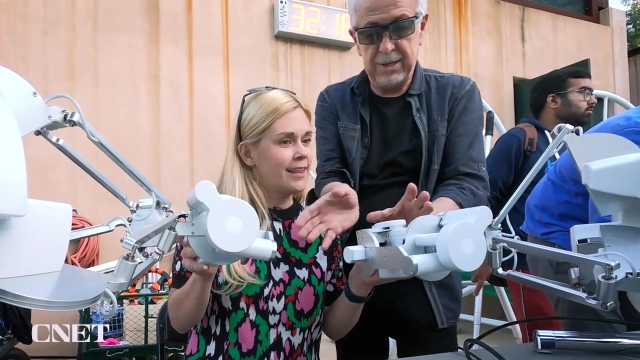 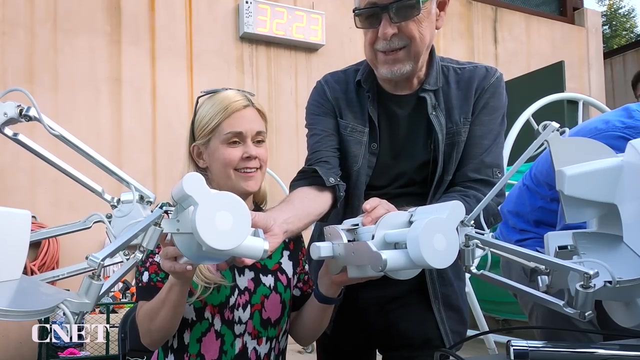 and you see the hands of the robot. Now they are your hands, You are moving them and you're coming closer and closer And I remember when I touched the Crispi, it was really, really emotional. The The Stanford swimming pool is a long way from the Mediterranean. 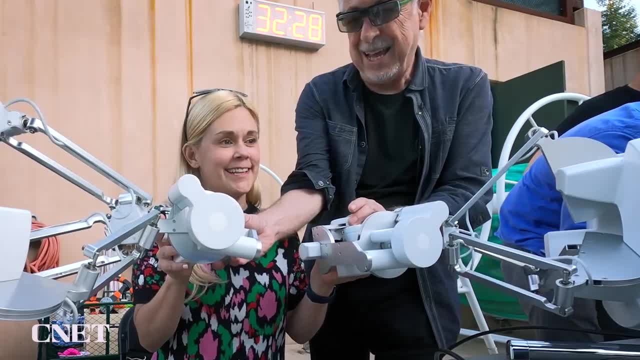 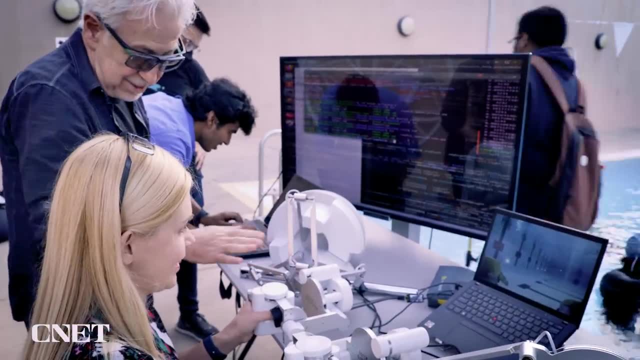 But here I got a great sense of what it feels like to operate this robot. You just go like a little like this, And when you want to go to the left you go like this of the controls and how to steer and move the robot underwater, and then it's. 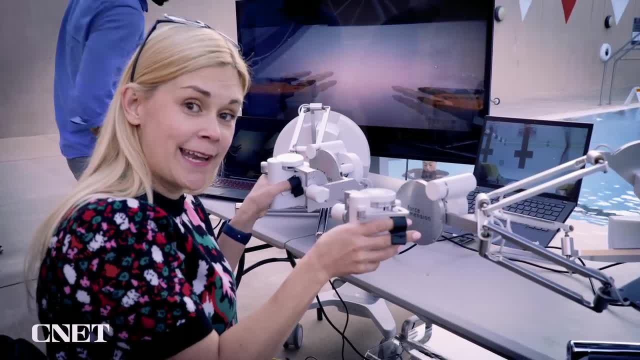 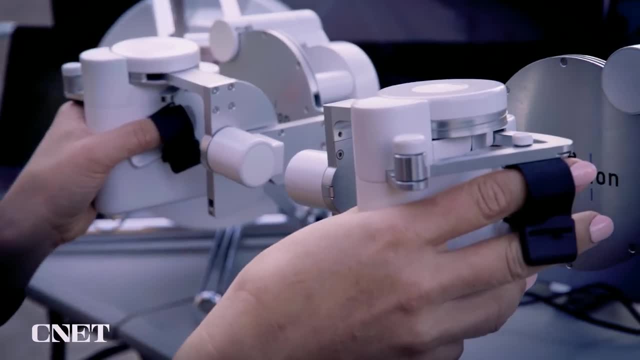 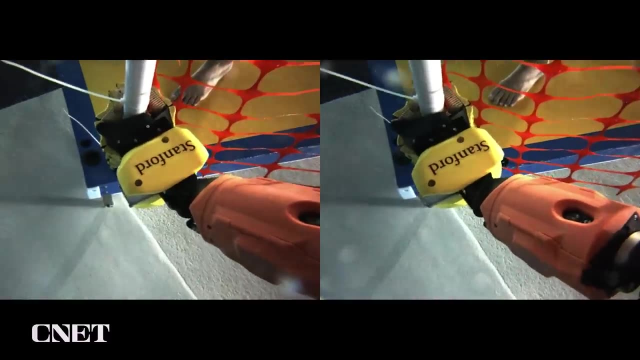 up to me. So, even though the robots in the water right now, I can actually control it with these haptic controllers and they're designed to be incredibly intuitive. so it feels as though you're moving your own arms, so I can squeeze in to grasp objects and the robot hands move, but also I'll feel resistance. so if 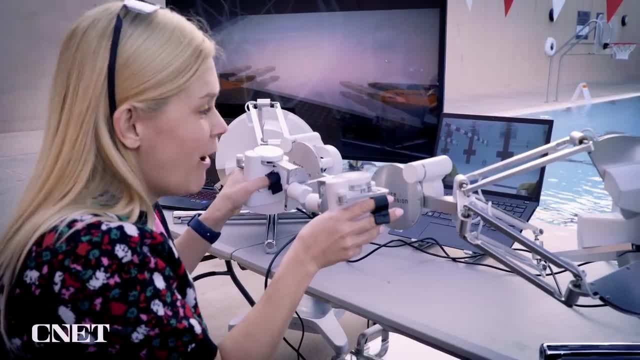 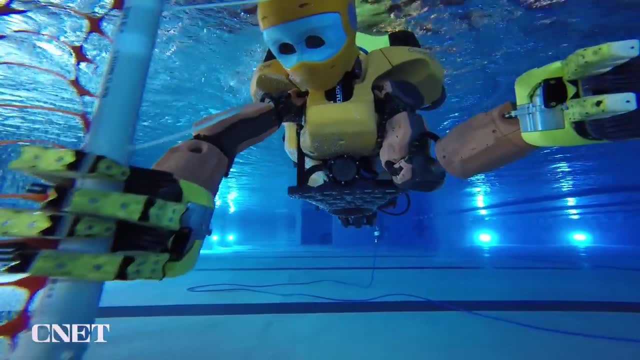 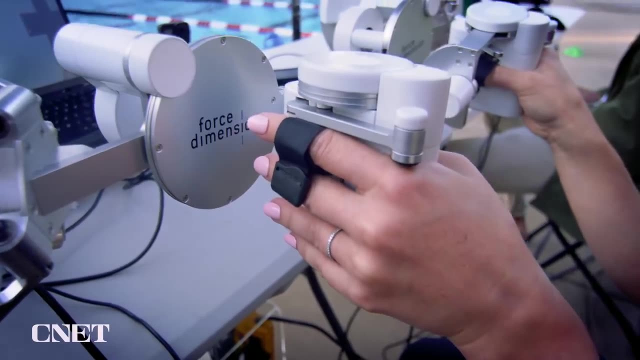 I run the robot into a wall, which I shouldn't do. I'll actually feel that feedback in these controllers. Even though the robots underwater, I'm still fully in control. Controlling the robot from the surface is one thing, but getting underwater with the Ocean 1K is a whole other experience. 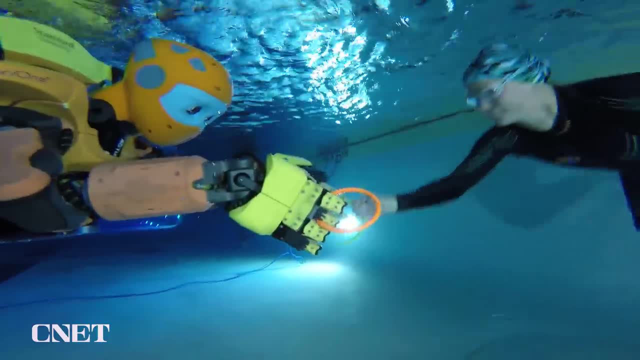 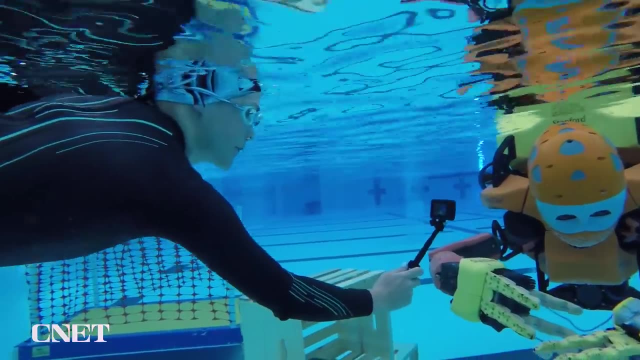 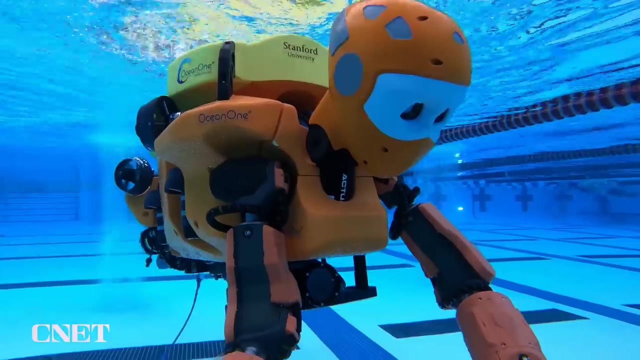 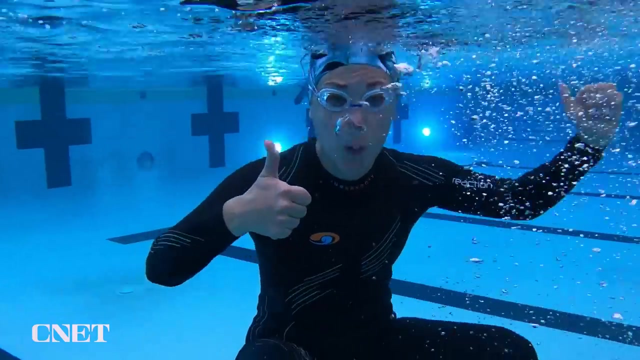 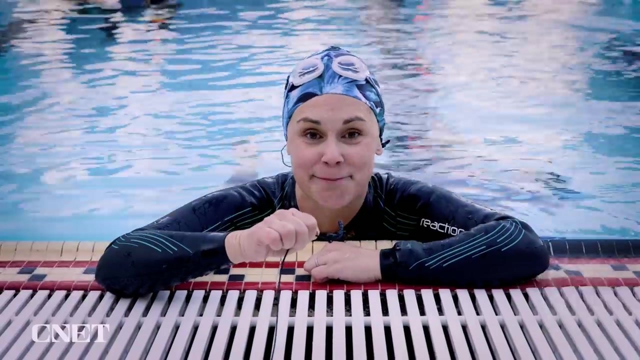 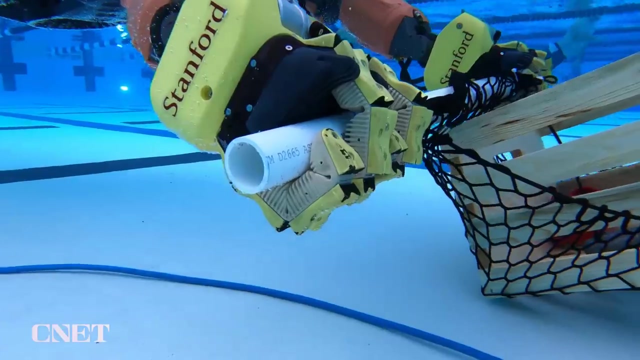 I just finished swimming with a robot. I've got mad goggle rings around my face, my eyes, but it's amazing. it feels a lot like swimming with a human. it's got eyes. it's got these arms holding things out in front of it. it's really surreal to. 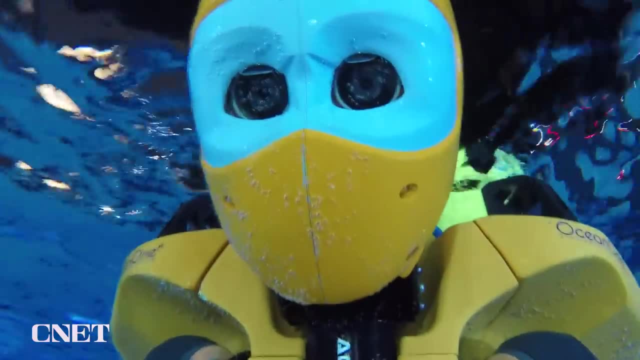 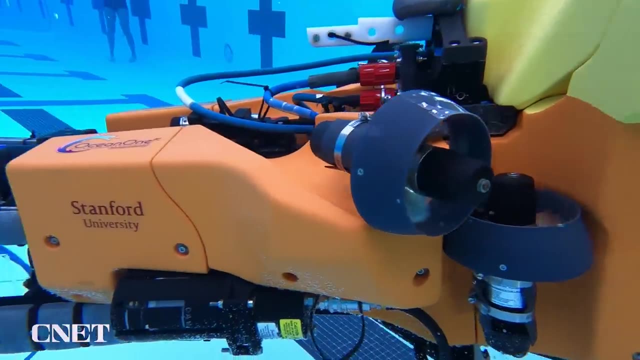 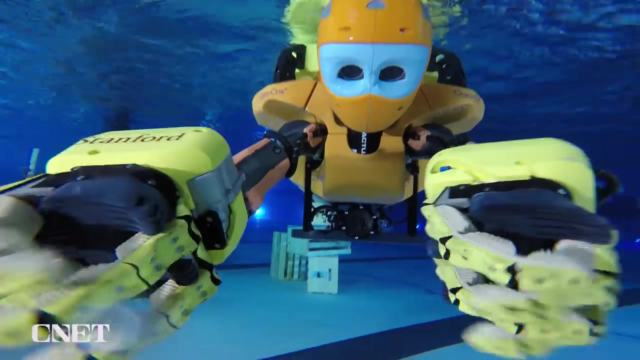 realize it's being controlled by a human, but it's also so robotic. I really agree with the engineers here. it feels kind of like your avatar under the water. you know I'm dealing kind of with a human, but it's still incredibly robotic. I kind of want to keep swimming with it. it's a bit like swimming with a dolphin, but way. 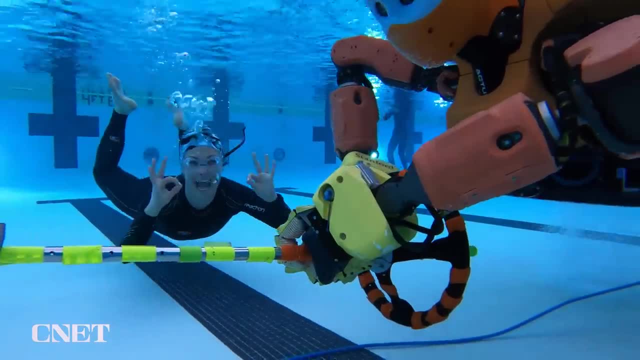 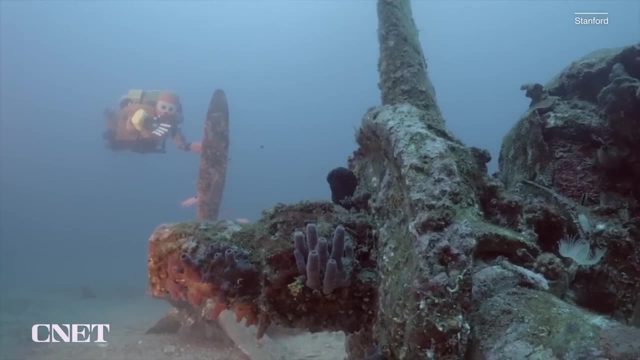 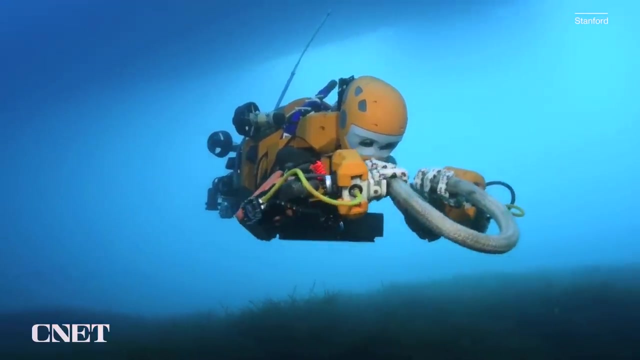 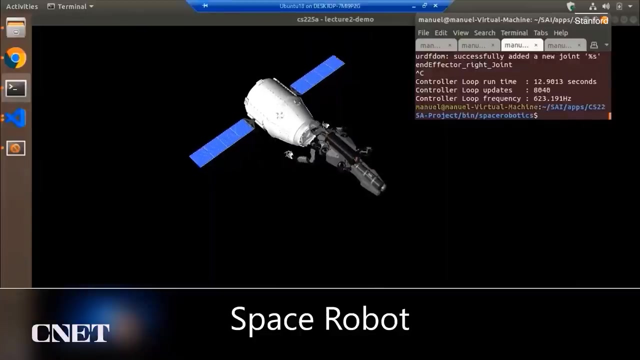 more high-tech. after swimming with the ocean 1k, it's easy to see how much this could change. underwater exploration, handling delicate coral, exploring shipwrecks, even commercial jobs like fixing underwater pipelines- anywhere. you need human dexterity, but you can't send a human. the ocean 1k might even one day. 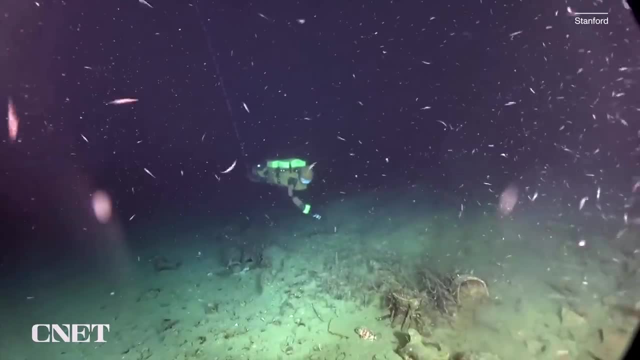 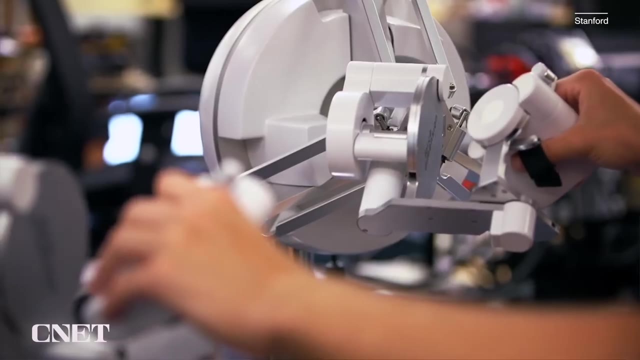 be used as a life saver in the future. Imagine a robot that could explore lakes on distant moons and exoplanets. for now, the Stanford team is still testing and improving the ocean 1k, whether it's in the deep ocean or in the Stanford swimming pool, after all, there's nothing.